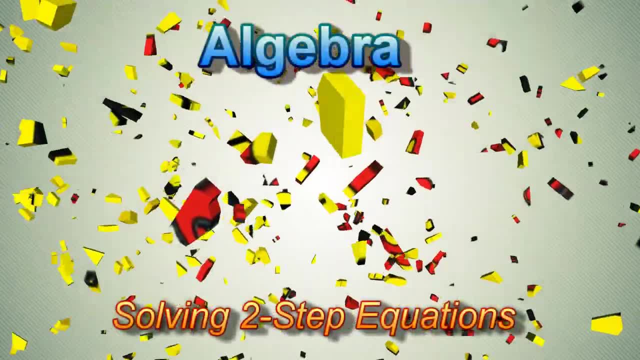 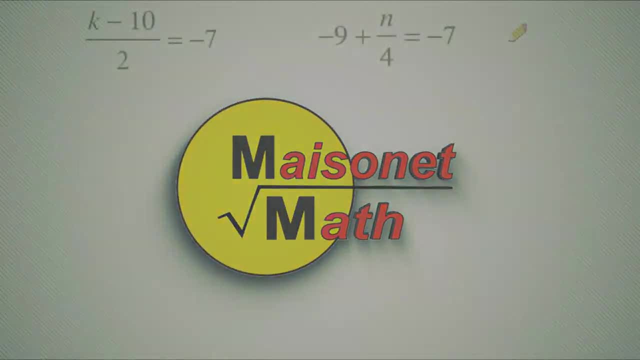 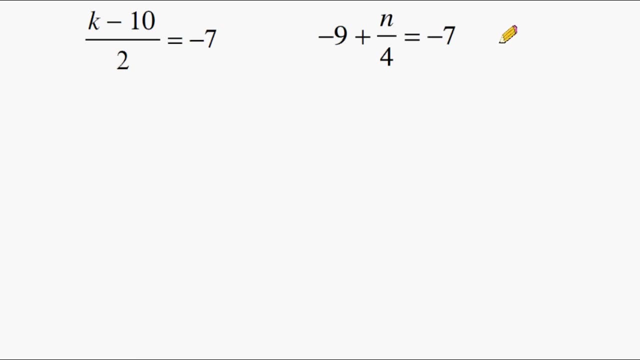 Alright, what we're going to do in this tutorial is practice solving two-step equations. Now we're going to do two examples, and the two examples are very similar to each other, but we have to do each one of them slightly different. If we take a look at the first example, notice. 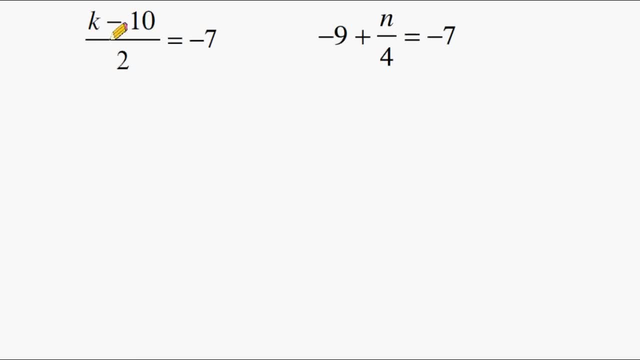 that one of the steps involved in the equation has a division operation, as does this one too. But notice, with this equation, right here we have a difference at the top, and then we're taking that entire difference and then dividing by two, but over here we don't have a subtraction. 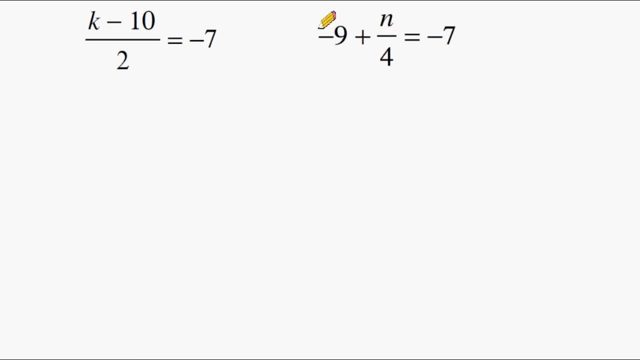 problem. as the complete numerator, We have a negative integer here and then after that we're adding a fraction, So we have to deal with each one of these slightly different. Now, when you have an entire difference or a sum as a numerator, what I like to do is: 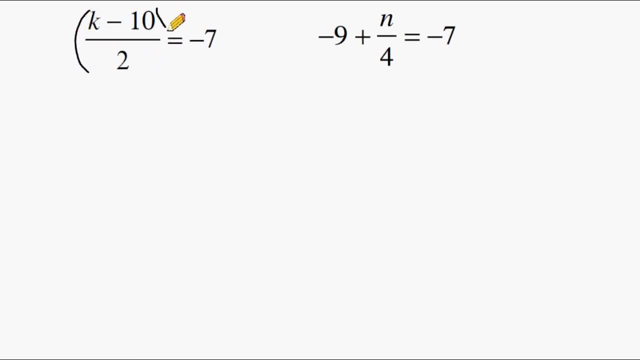 put parentheses around the entire quantity, like this, and because we're dividing by two, we take what we're dividing by, or the denominator, and then write it as a numerator. Now, what that allows us to do is this: It allows us to cancel out this number right here on the 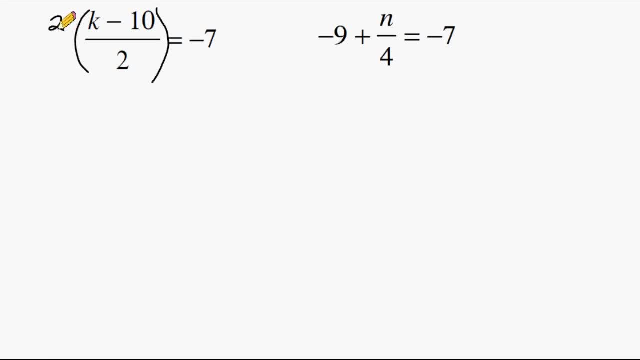 left-hand side of the equation. So it's kind of like this: A whole number like two can be written as a fraction, So that's like two over one. So basically we're taking this entire quantity, which is a fraction, and multiplying it by two over one, which allows us to cancel out that denominator. 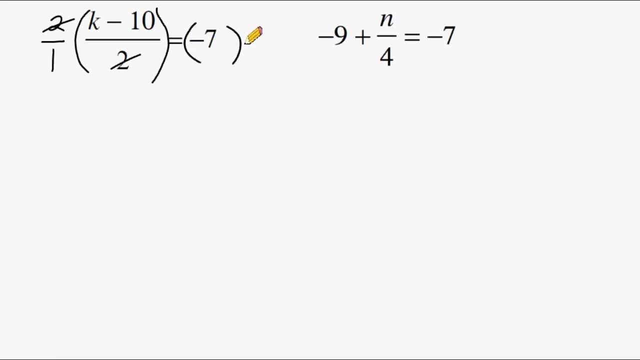 And then we take the other side of our equation and we multiply by that same number. So we just take that denominator, write it at the top so it cancels on the left, and then multiply it on the right-hand side. And negative seven times two is negative fourteen. 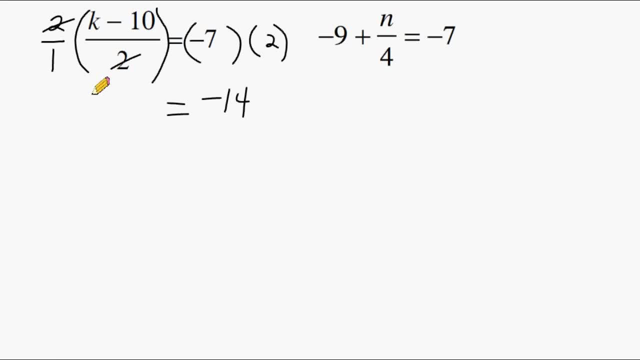 Now, because we canceled out this two. that leaves us with K minus ten on the left-hand side of our equation, And then we just do the inverse of minus ten, which is to add ten, And what we do on the left, of course, you've heard that a million times we have to do. 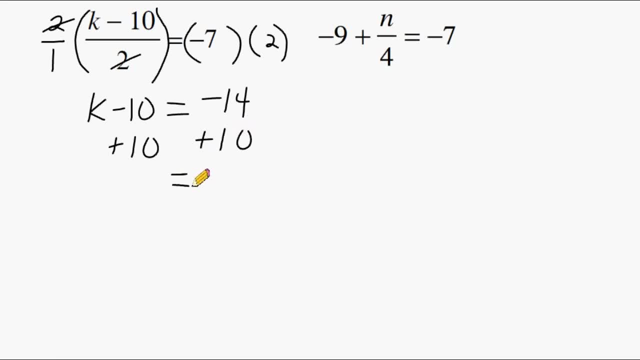 on the right-hand side. Ok, so on the right-hand side now we have negative fourteen and positive ten, which results in negative four. On the left hand side, opposite integers result in negative four in 0, and k plus or minus 0 is just k, so we just have k equals 4.. I'm sorry, I. 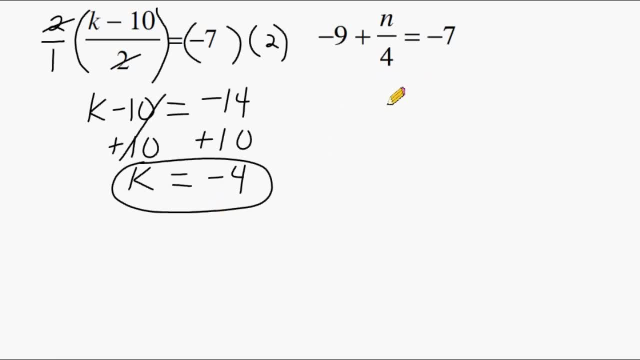 should have said: k equals negative 4.. Now, on the right hand side, we have to approach this one a little bit differently. So if you have a number separate than your fraction, you've got to start by doing the inverse of that integer first. So we're going to do the opposite of minus 9, which is plus 9.. So 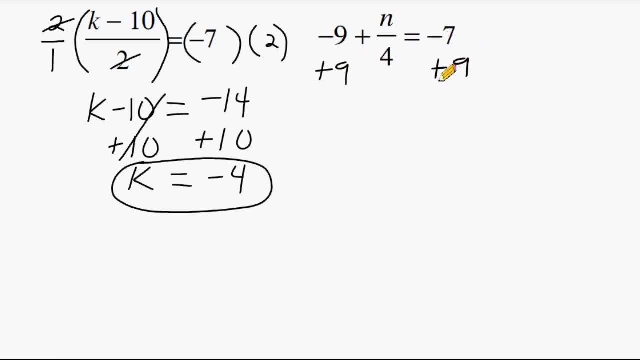 we have to add 9 on the right hand side of our equation. Negative 7 and positive 9 results in positive 2. These opposite integers cancel on the left, leaving us with n divided by 4.. And now what we do is we multiply both sides by 4, because 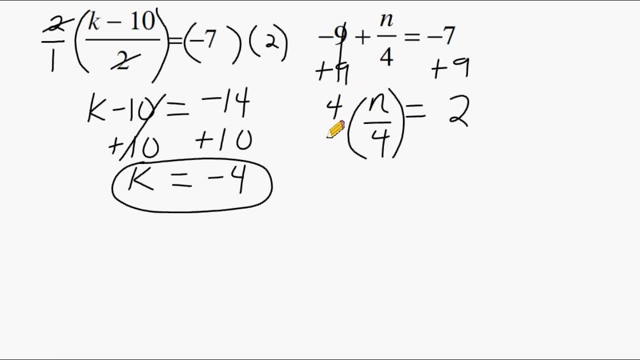 the inverse of dividing by 4 is multiplying by 4.. Now we really only have to write that denominator as a numerator So they can cancel out. But keep in mind, it's really like multiplying 4 over 1, but we do not have to write that one at the bottom, So we cancel out the 4's. 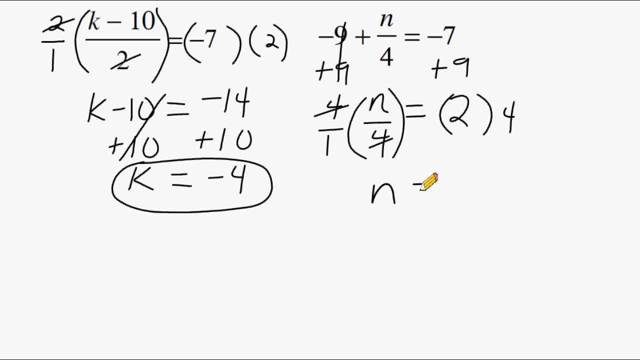 That leaves us with n, and on the right hand side we have 2 times 4, which is equal to positive 8.. And of course, if we want to verify that these answers are correct, we would plug these integers in to the variable, into the original. 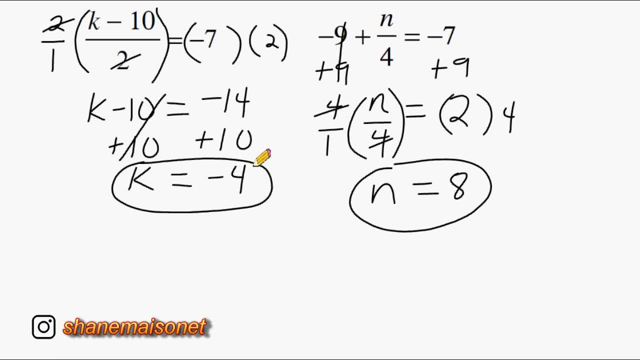 equation. So let's go ahead and do that really quick. Up here we have k minus 10, so we have to replace this k with negative 4.. So negative 4 minus 10.. Then we have to divide by 2 and that should be equal to. 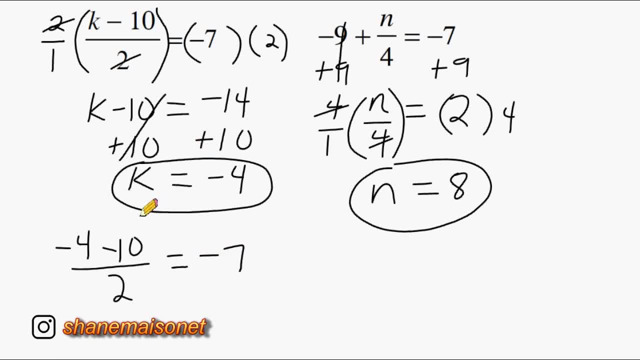 negative 7.. Negative 4, negative 10 is negative 14.. And negative 14 divided by 2 is in fact negative 7.. So that one does check out. Now over here we had the equation plus n over 4 in n we came up with is equal to 8, so we're gonna write 8 over.